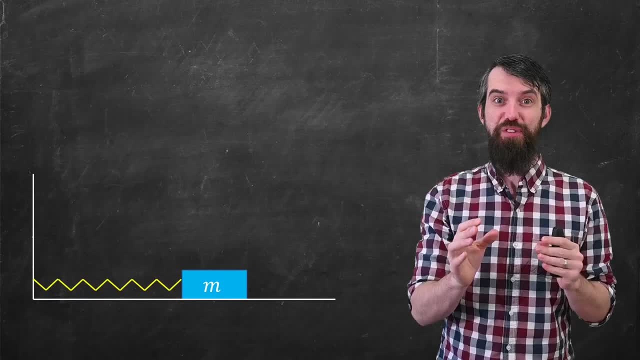 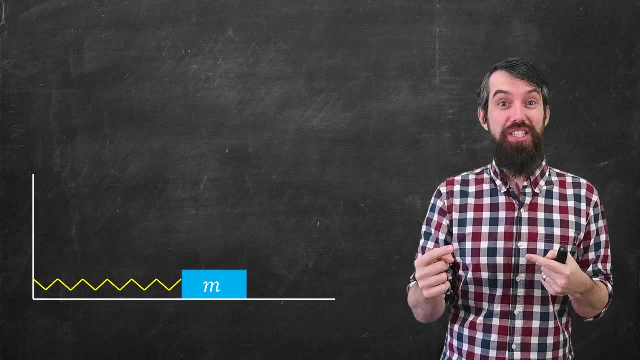 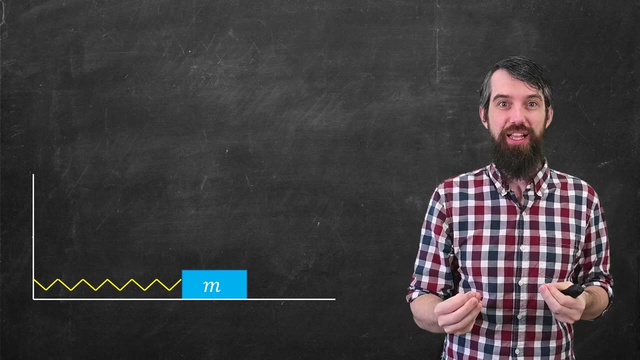 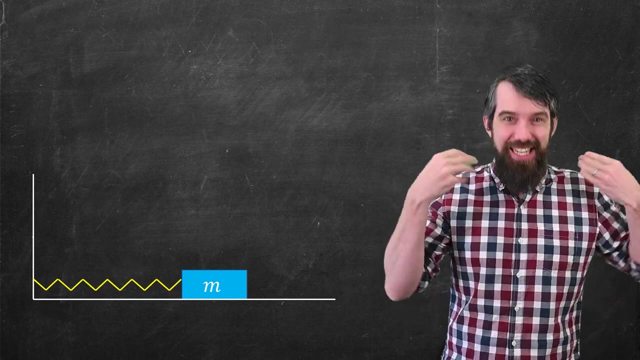 In this video we're going to talk about mechanical vibrations: a mass going back and forth on a spring. This kind of motion is sometimes called harmonic motion and is incredibly important throughout physics with a wide range of different types of applications. So what's the idea? I want to imagine I have a mass M it's sitting on some surface which, at least at the beginning, I'm going to presume is a frictionless surface. 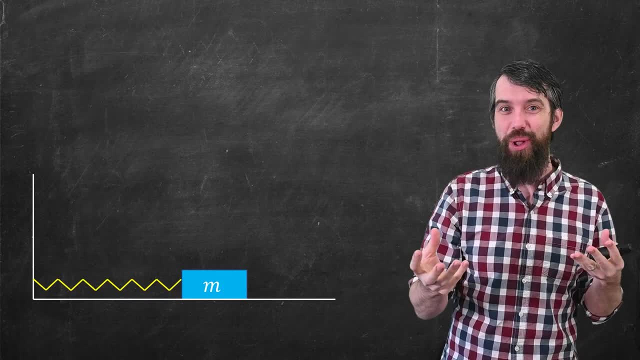 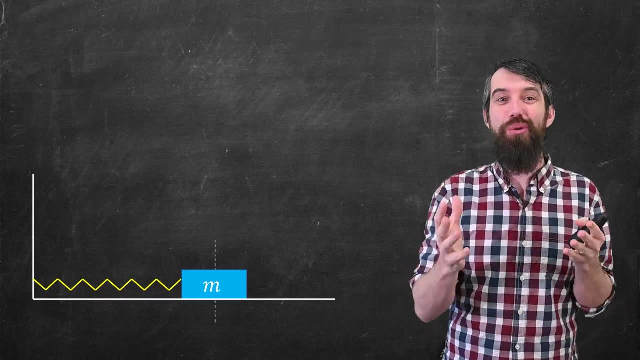 Maybe it's ice, or maybe there's really nice frictionless wheels in the block, something like that, and it's attached to a spring. So if at the beginning this is at rest, for example, I'll put an equilibrium position to say, if I don't touch anything, that would just sort of rest right here. 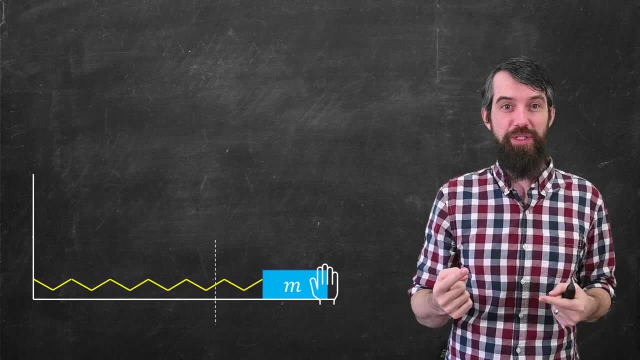 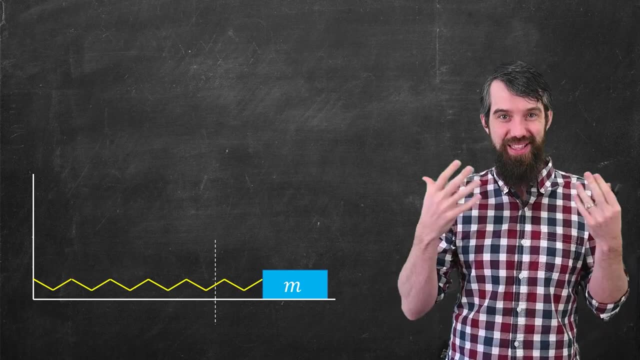 But if I grab it, I could move it away from that equilibrium spot. And then the question is: well, what happens if I let go? Because it's a spring? the spring is going to want to return it to the equilibrium position, but it can't do it directly. 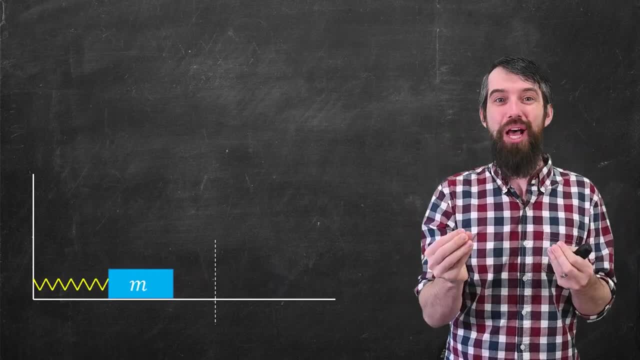 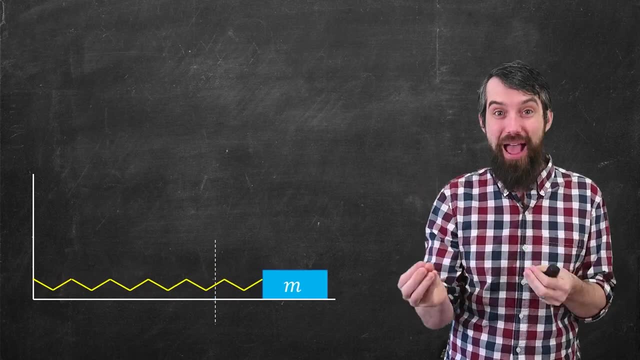 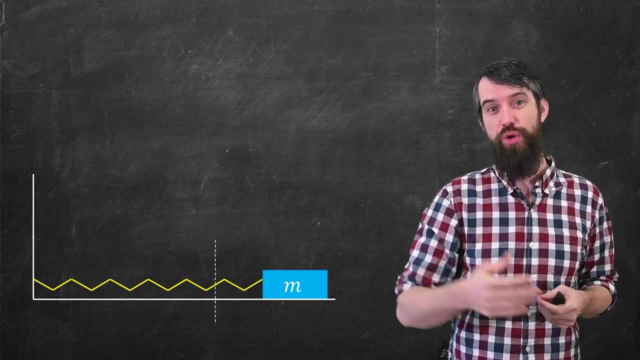 It's going to sort of go off and overshoot and end up on the left side of that equilibrium position And then you can imagine it would spring back and it would cross back over and back and forth it would go. So how do we model this? How do I write down equations that represent this? How do I solve those equations? 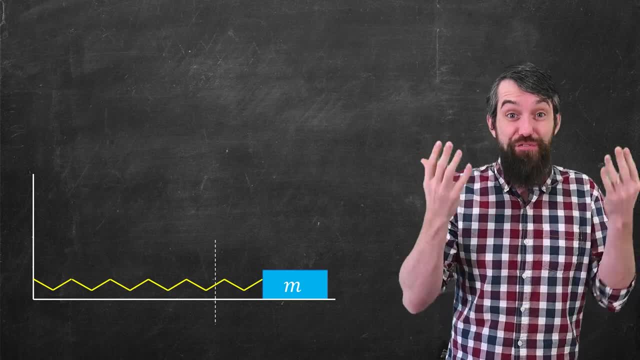 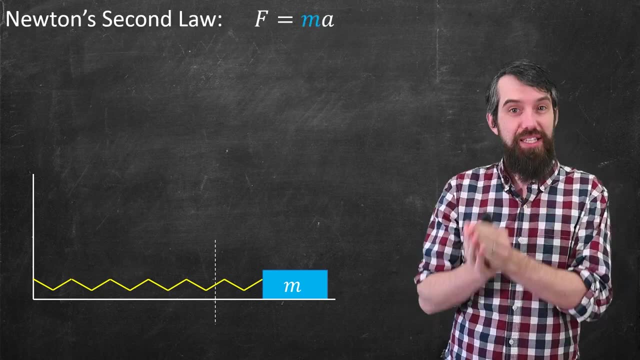 So we're going to begin with just a little bit of analysis of the forces that are involved, because we have Newton's Second Law that tells us that the sum of the forces is equal to the mass times, the acceleration, And it's going to be convenient for us to write. 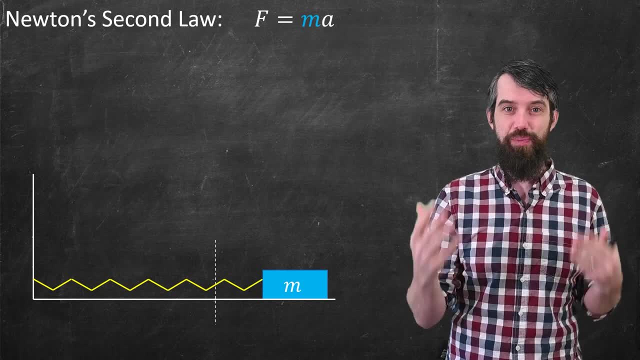 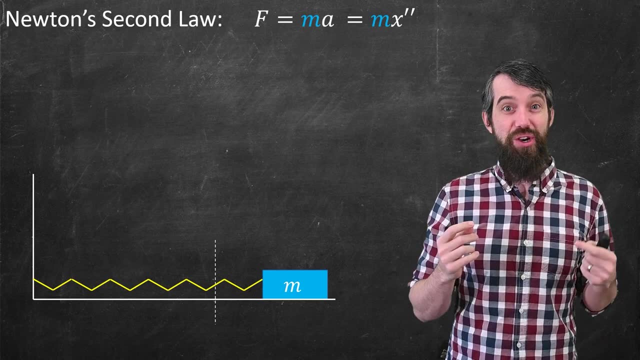 acceleration as just the second derivative of the displacement x. Now, the only force that's relevant- because I'm assuming it's frictionless at the beginning- is what we call Hooke's Law. And Hooke's Law gives us the force of the spring acting on the mass. 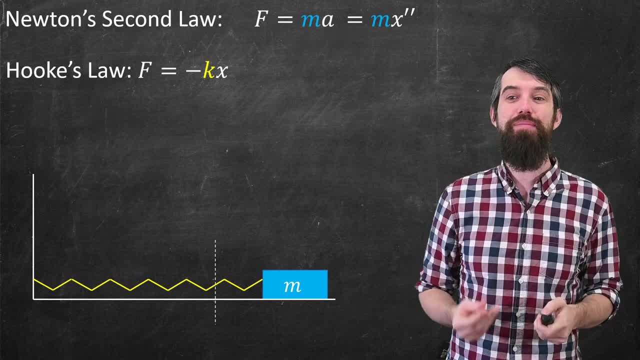 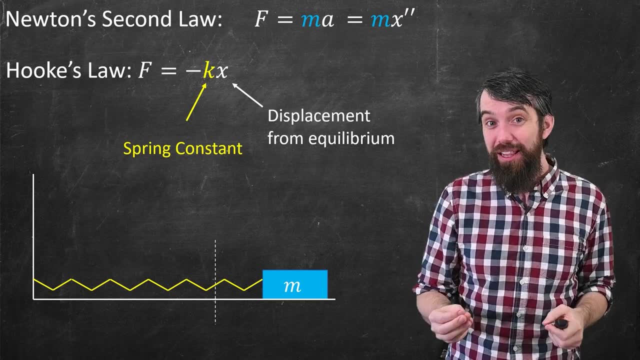 And the idea is it's negative k times x, where k is just some constant, And then x here I've represented as the displacement, but specifically it's the displacement from the equilibrium. So I have this one vertical line here which was 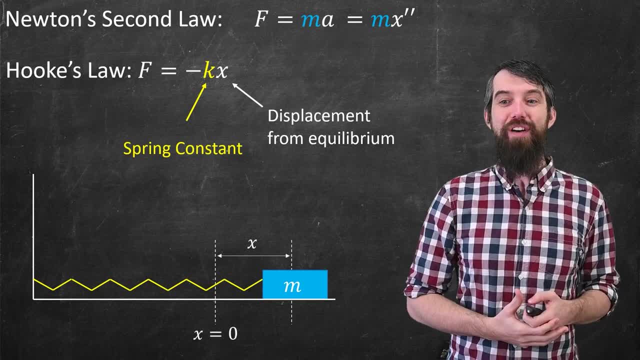 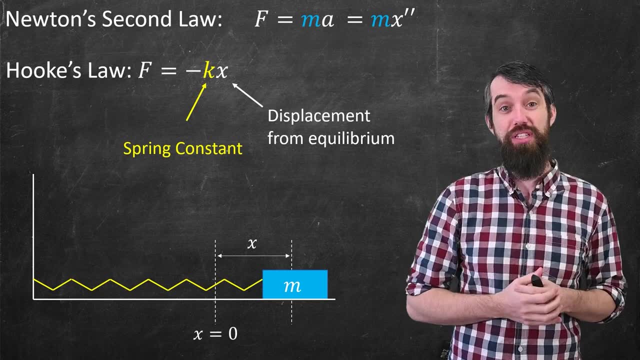 where the spring would like to be at rest. And if I move away from that, I get a displacement of x from x equal to zero, being that equilibrium position. That's the x that we're measuring specifically in Hooke's Law, And it's negative because if your x was to the right, if it was a positive value of x, 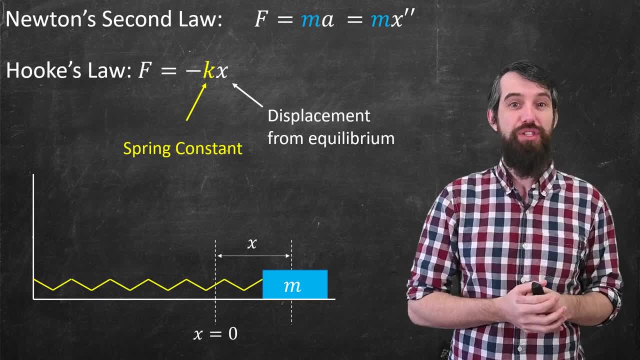 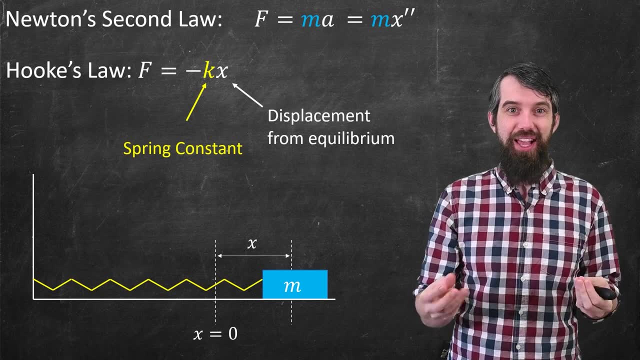 the force would push it back to the left. It would push it back towards the equilibrium point. So there's always that negative. And then the k, the spring constant. well, it depends on the properties of the spring. You've got really thick coils. 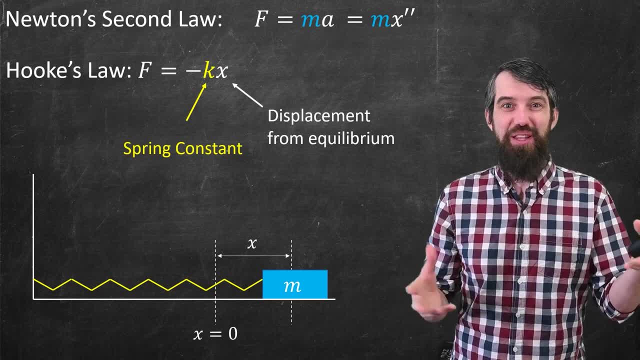 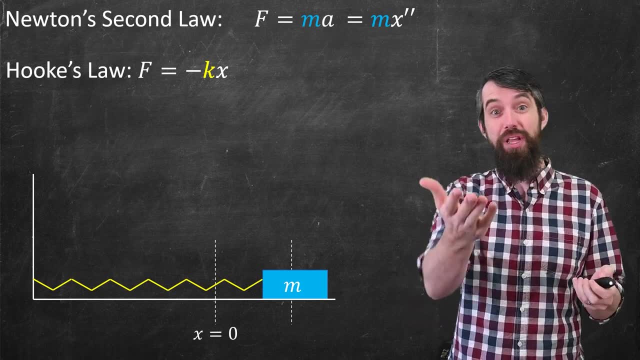 then you might have a larger value of k. a really light sort of flimsy spring would have a small value of k. So I have the generic Newton's Law for forces being mass times acceleration. I have Hooke's Law and I'm going to compare those two things. 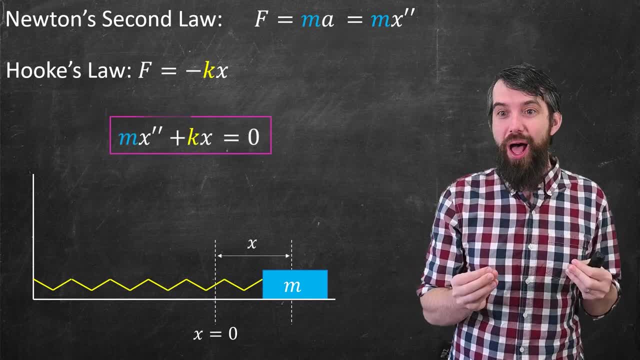 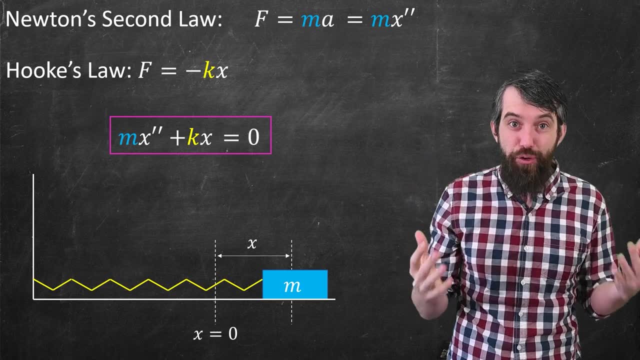 I'm going to say thus that mx double prime plus- because I moved the force to the other side- plus kx is equal to zero, And that is my differential equation to describe this mass on a spring. So now this just turns into a problem of solving differential equations. 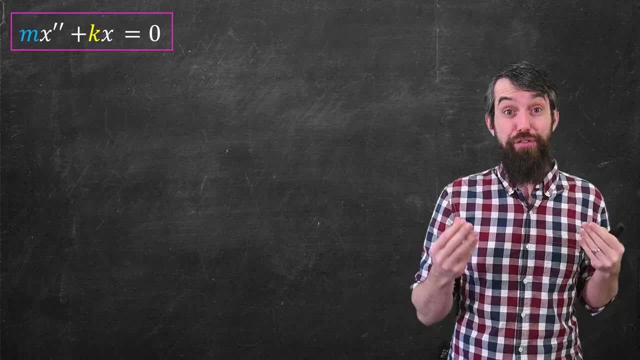 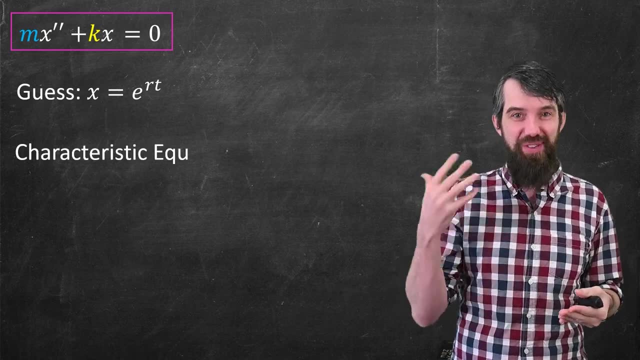 We know what to do. I'm going to guess a solution of the form. x is equal to e to the rt. for some unknown r. I get the characteristic equation because two derivatives of e to the rt gives me an r squared. So, mr squared minus k, cancel, the e to the rt's is equal to zero. 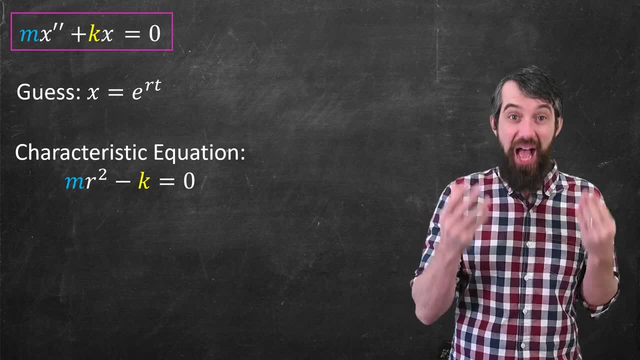 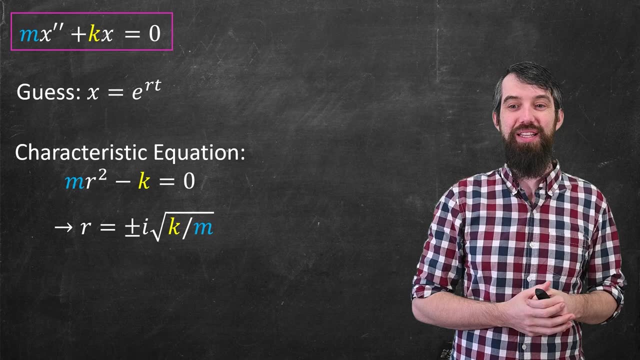 And then this I can solve. This is: r is equal to plus or minus. i times square root of k over m. The only thing that I'm going to do that's new here is I sometimes like to relabel this square root k over m. it comes up a lot. 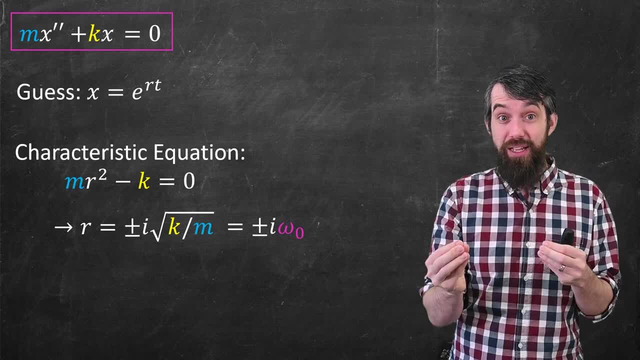 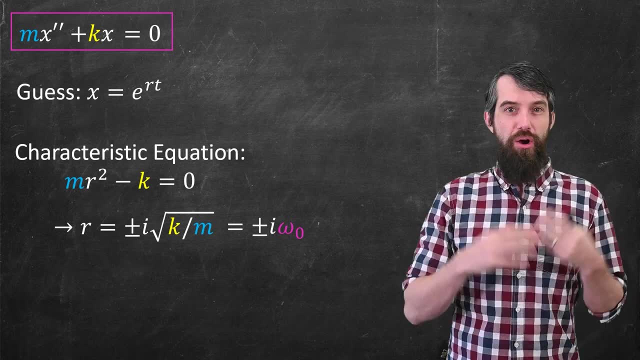 Sometimes this is re-labeled as omega naught. Omega naught here just stands for basically the frequency, as I'll show you in a little moment. So it's just a shorthand for root k over m. Okay, so what was the next step in our process to solve a differential equation like this? 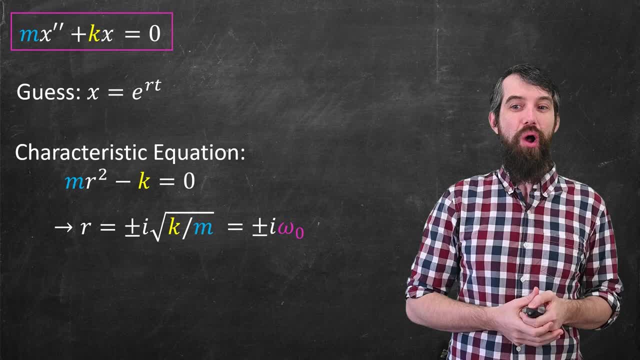 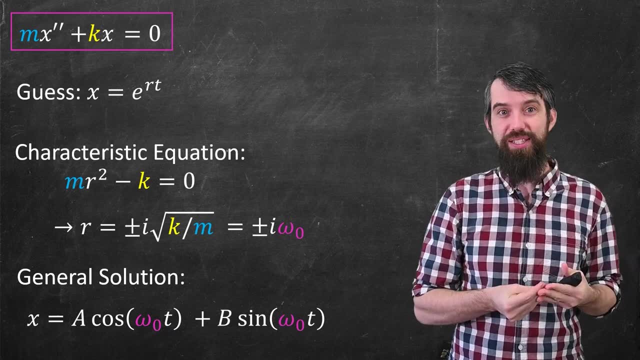 Well, e to the plus or minus i omega naught we saw could be converted into sines and cosines. There's no real part to our r's, so there's no exponentials, And the imaginary part by Euler's formula gets converted to cosine and sine. so I get a cosine omega naught. 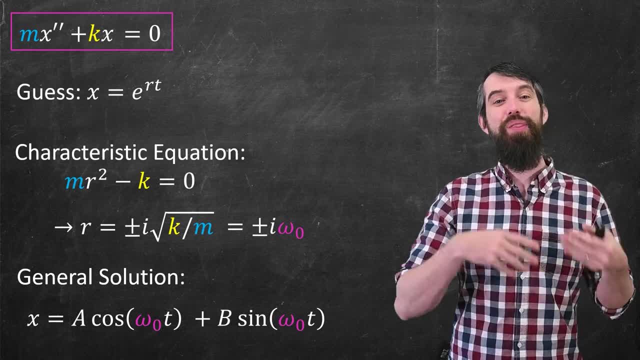 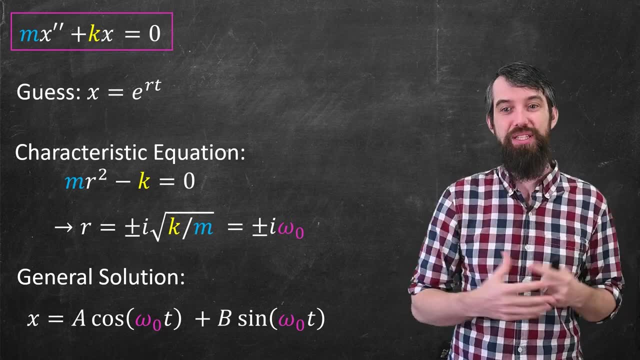 t plus B sine omega naught t, And it's in this context that it makes sense to call omega naught a frequency. It's cosine omega naught- t, and thus I get the frequency of omega naught. Bigger value of omega naught means my sine and cosine terms oscillate faster. 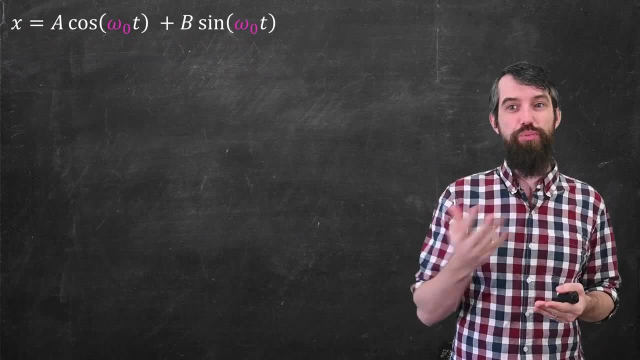 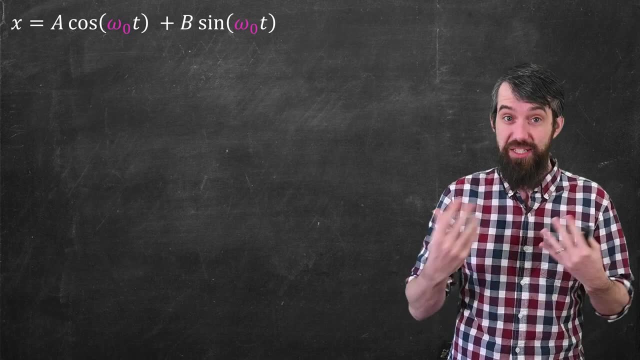 So this solution that I have to the mass on the spring problem is perfectly fine and it does make sense from the perspective of oscillations. Cosine and sine are both oscillating terms And we were expecting our mass on the spring to go back and forth and to oscillate. 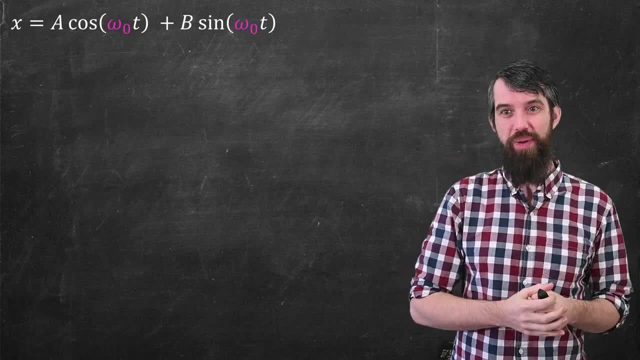 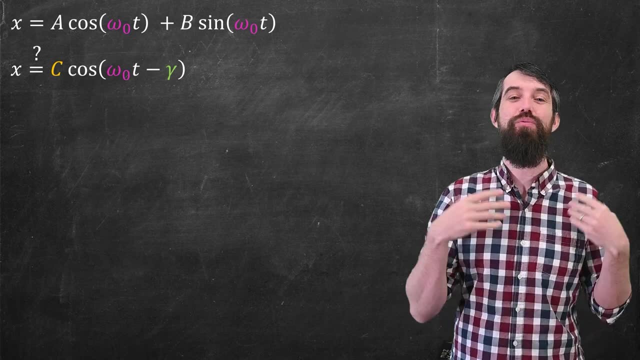 But there's one other standard little trick that we do here, because having a cos and a sine is a little bit annoying, So I want to combine them. I'm gonna see whether it's possible for me to write it in a new way. 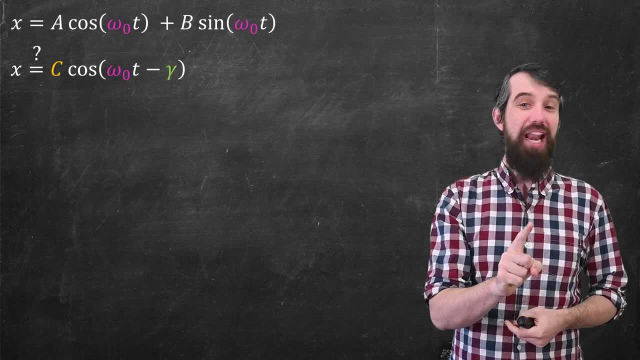 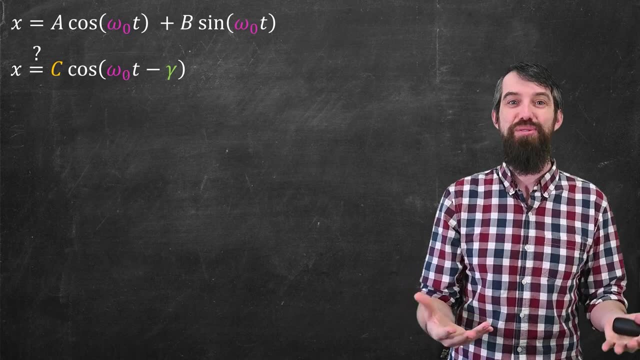 which is with only one trigonometric term, cosine. So I can have a new coefficient, co, at the front, and then I'm gonna have the omega, naught t, but then minus a gamma. So I haven't showed you how to do this. I'm gonna see can I do it. 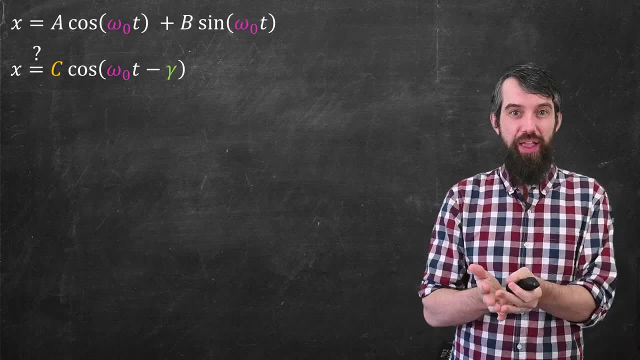 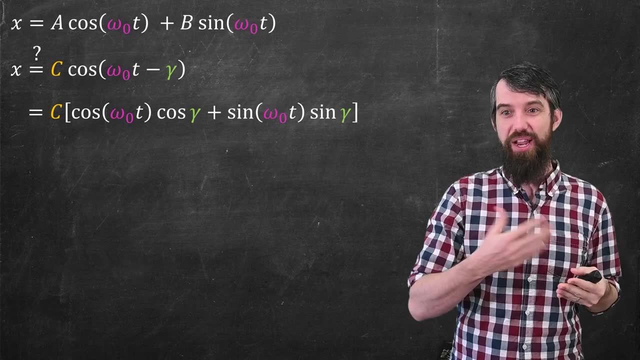 Well, we have a trigonometric to deal with: cosine of one thing minus another thing. So I could expand that guess and write it as the constant co at the front, then cosine of omega naught times cosine of gamma, and then plus sine of omega naught times sine of gamma. 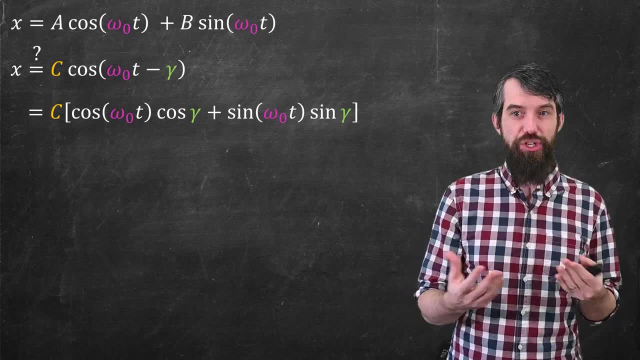 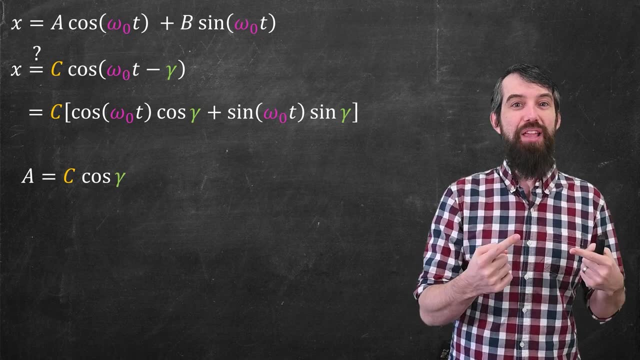 So if I compare this to the original, well, for example, there's a cosine of omega naught t in both two places, but I get these relationships that a then would be c times cosine of gamma and b would be c times sine of gamma. 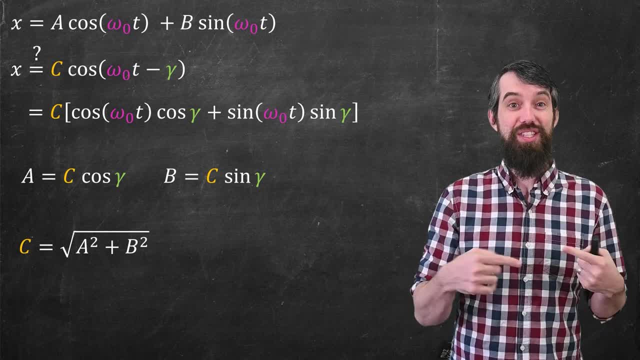 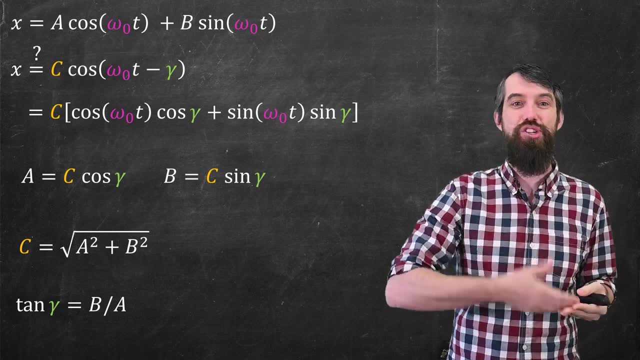 And now it's just a question of solving for everything. So for example, I can solve for the c just by Pythagoras- It would be square root of a squared plus b squared. and I can solve for the gamma, because the tangent of gamma would be equal to b over a, and then you could take an r-tan from there. 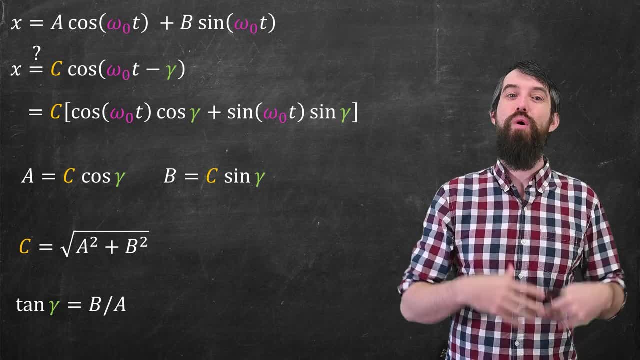 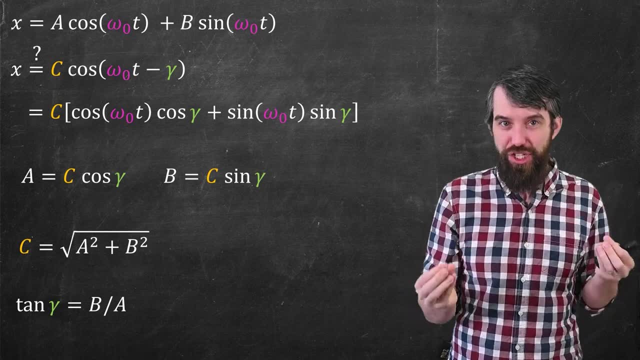 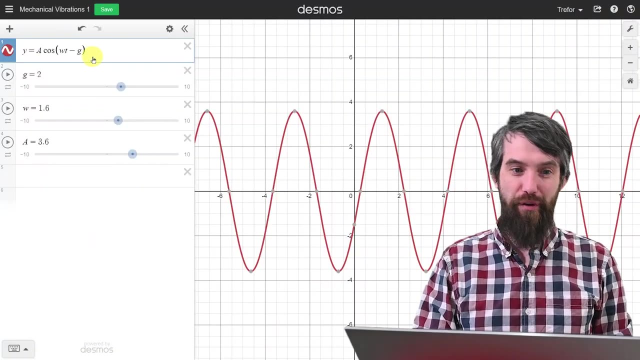 And so the final point is that this solution of the form- a number c times cosine of omega naught t minus gamma- is really the solution to the frictionless mass on this frame. Let's check out what this looks like graphically. Tell me graphists I've come and put in this function of the form. 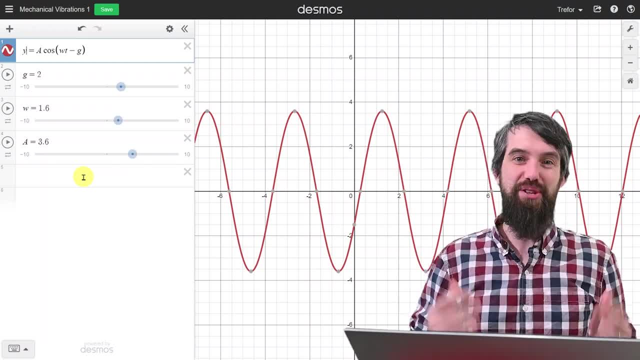 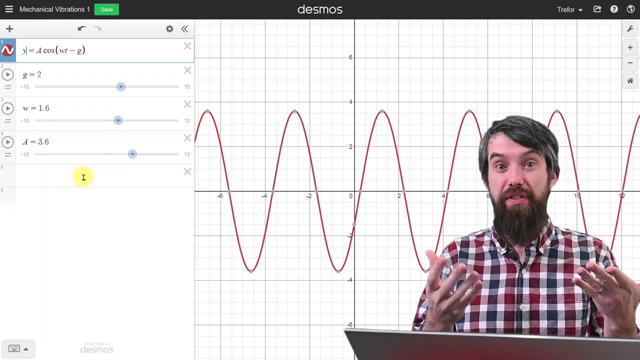 a cosine Wt minus g. I have to use Roman numerals, not Greek ones, for this particular software, And what I'm really interested in is: how does the shape of this curve change as I change the different parameters? And first of all, we see this sort of oscillatory behavior, and that is. 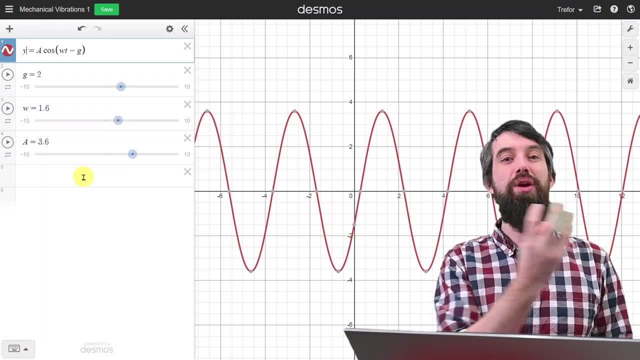 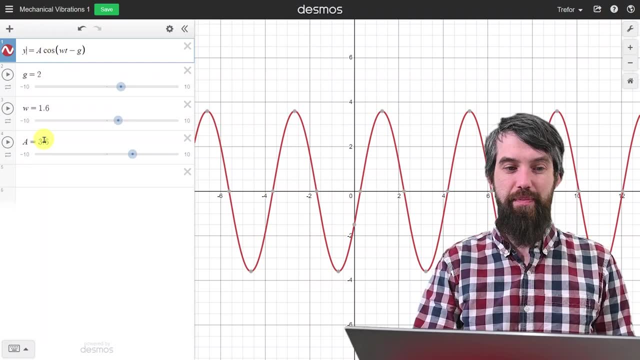 corresponding to, if I think of y as my position, this mass on the spring going back and forth and it's oscillating, so that at least makes sense. The coefficient a out the front here is represented by amplitude and I can grab this slider and change it, and if I make a bigger value of a I get a bigger amplitude, and if I make a,